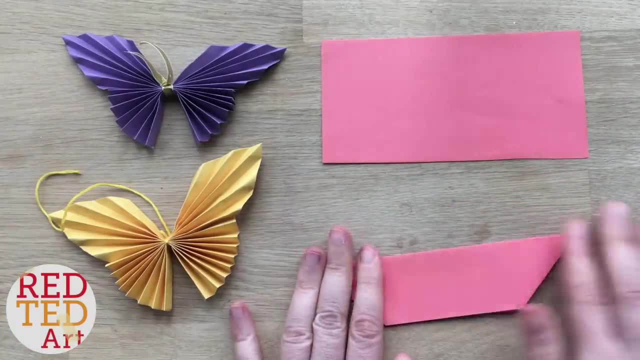 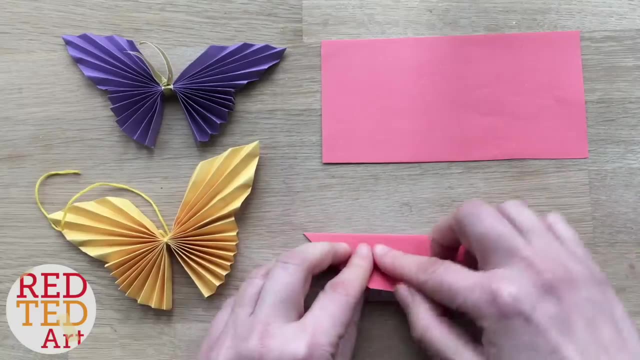 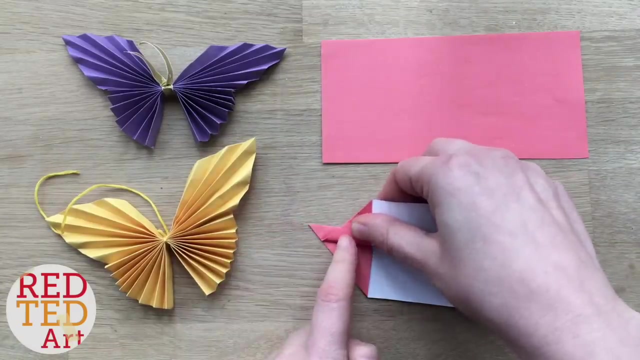 folding. it is quite nice. Now I'm just going to fold these again. So now what you need to do is create this concertina effect. So I'm going to fold my bottom piece up to about half a centimetre's width, So this bit that's left here is half a centimetre. Get it as straight as you can and to 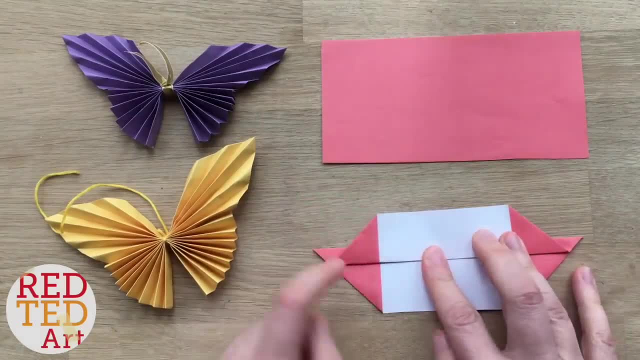 be honest, it doesn't have to be exact. So I'm going to fold it up like so, and then I'm going to fold it up exactly half a centimetre. It's an approximation, okay. So when you fold it over, you can see this. 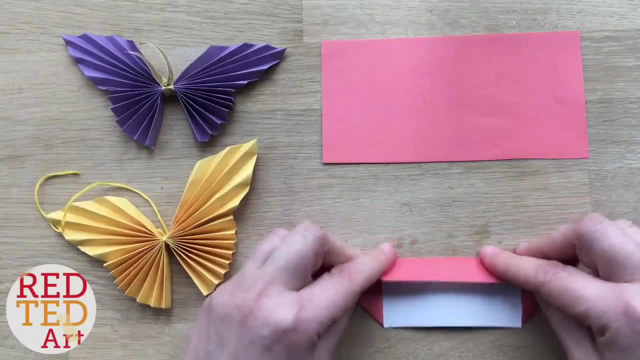 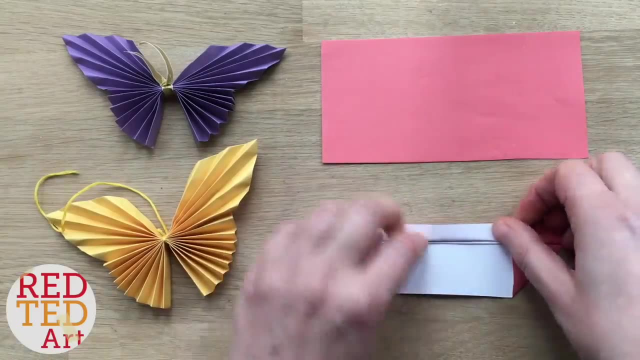 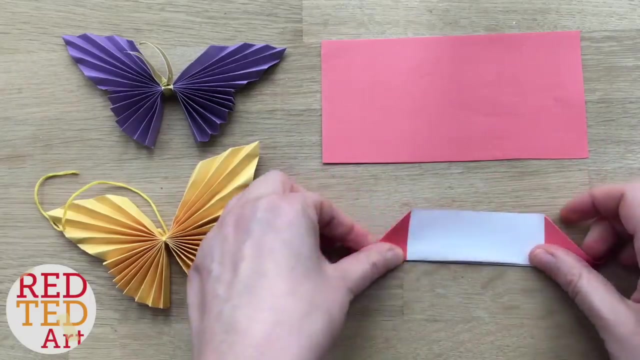 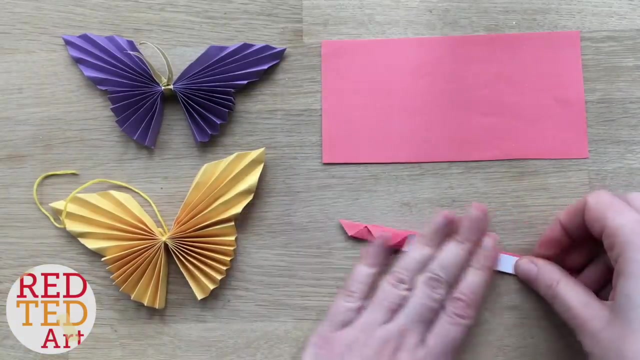 fold here. Now you fold it down again like so, and then you fold it up again like so: Right, and then you repeat the same on the other side. So basically, you're concertina-ing your paper around that central line. See, mine isn't super neat. 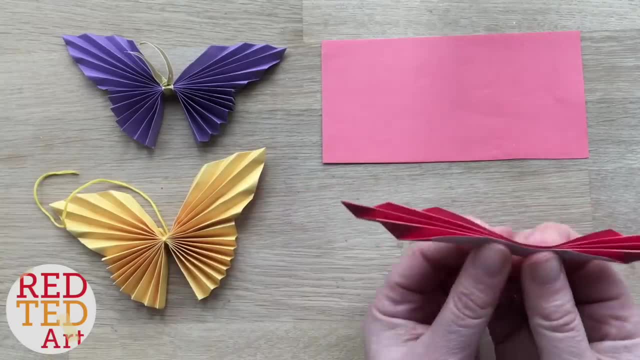 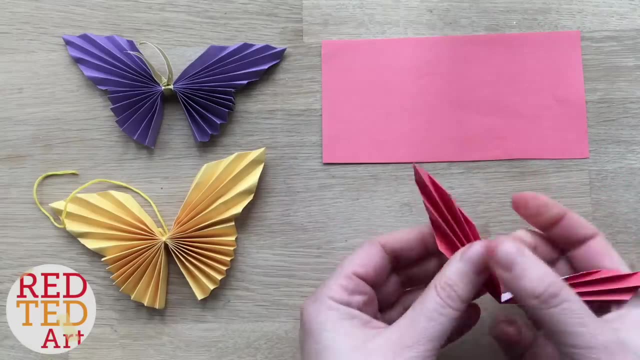 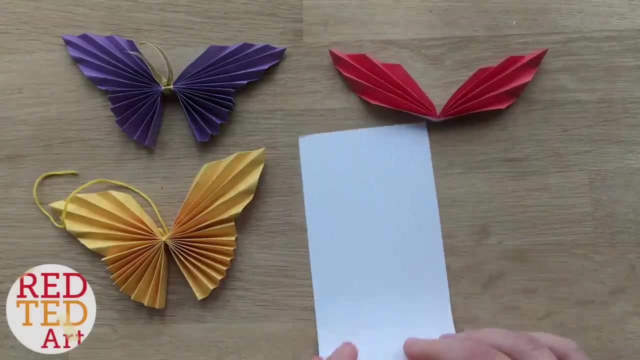 but it will still look cute. There we go Now. fold it in half like so, and you've got your top half of your butterfly. Now the great thing about this is you don't have to use origami paper. You can use any paper you've got, and you can basically recycle magazines and the like. So now you want. 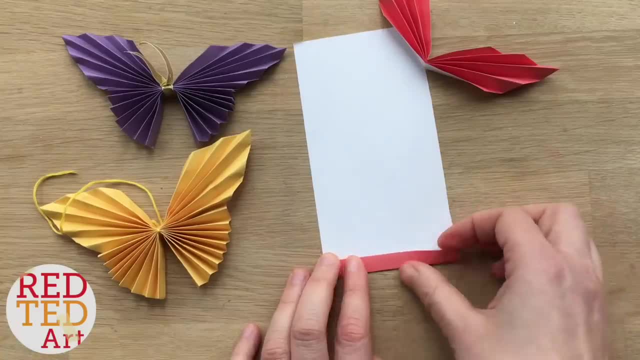 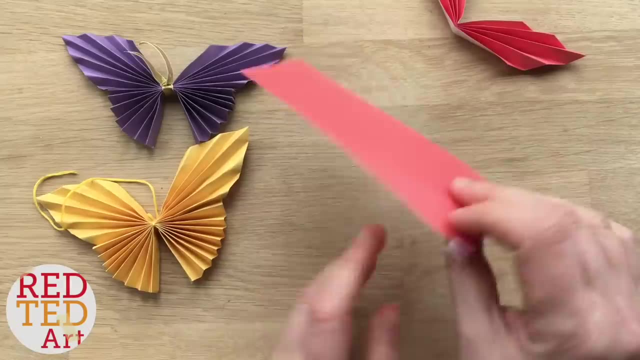 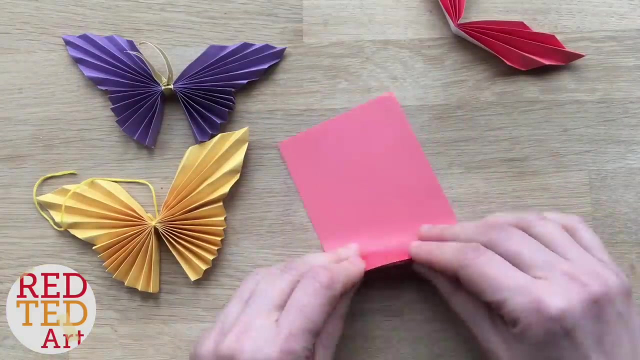 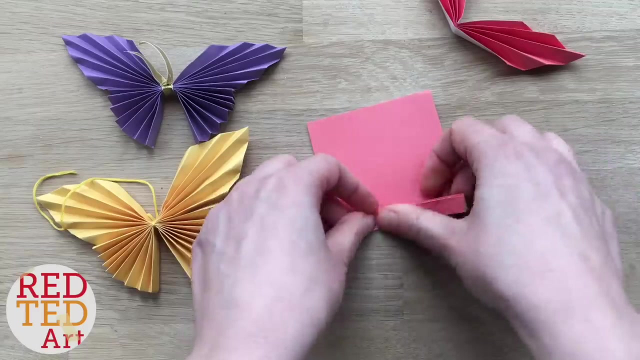 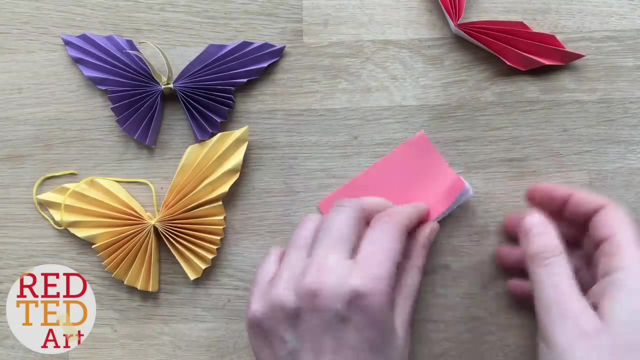 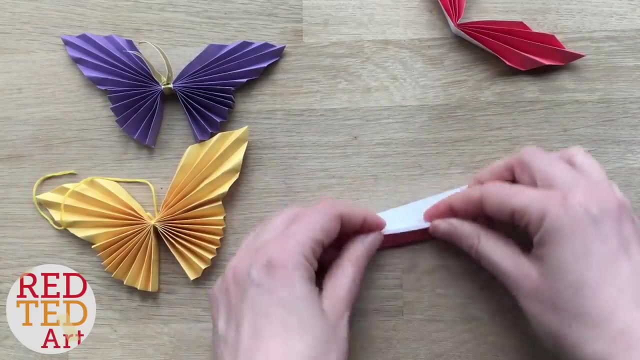 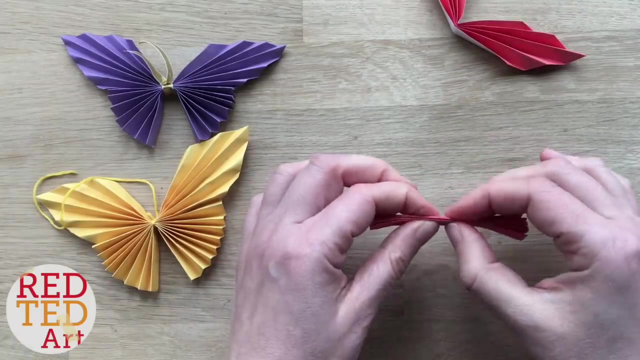 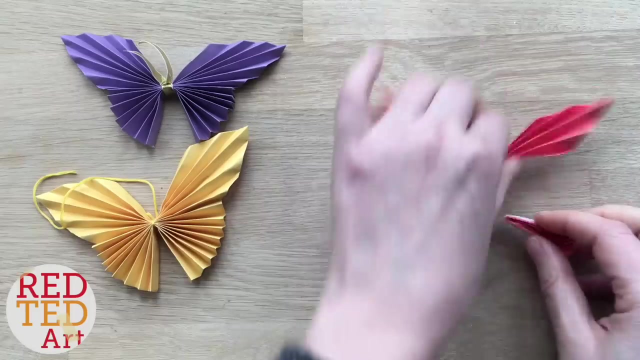 to do basically a concertina up that way in the same distance. So a half a centimetre Hunh. there we go. now you need to fold it in half, like so, and then you need to connect your two pieces. now, if you wanted to, you could add a little bit of glue here, but it's not strictly speaking. 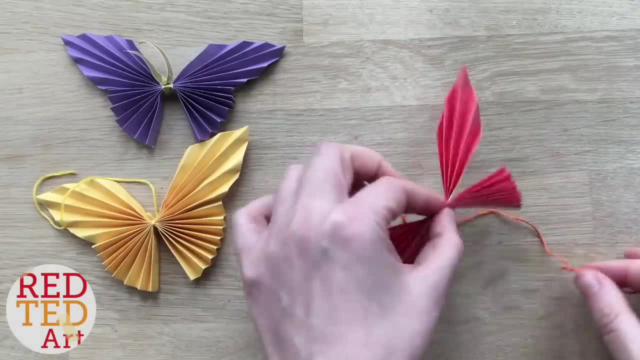 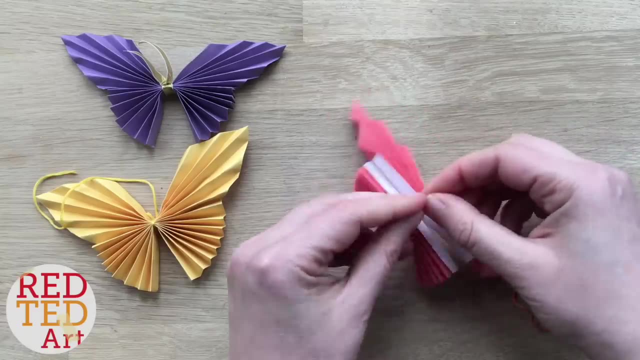 necessary. but you know, I think it's fine that what I'm going to use is there's a little bit of embroidery thread in a similar color to my paper. now, if you don't have embroidery thread, you can use normal thread, you can use pipe cleaners, you can use ribbons, like I've done.